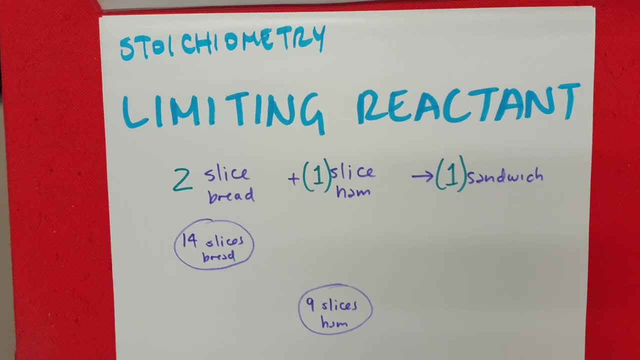 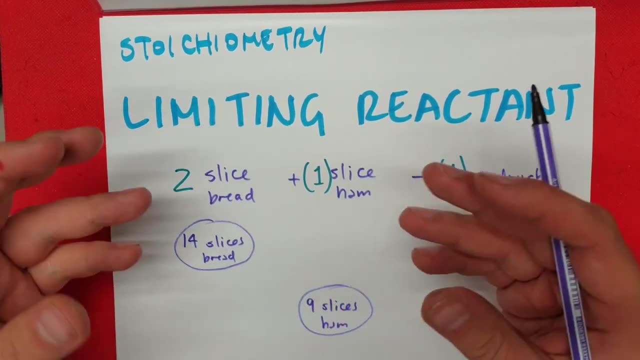 is what we actually have in front of us, right? so this is very simple to understand. if we have 14 slices of bread, how many slices of ham do we need? well, we know a sandwich, right? two pieces of bread, one piece of ham. so if I have 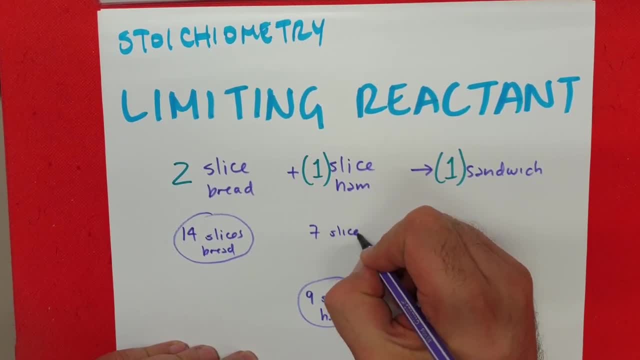 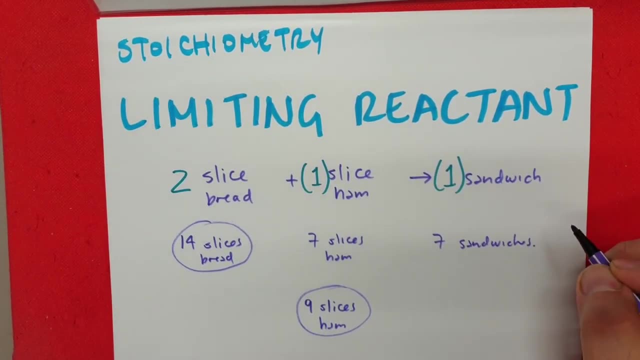 have 14, I'm going to need 7 slices of ham, And that would allow me to produce 7 full sandwiches. However, I'm given 9 slices of ham. If I need to use all those slices of ham, I would need 18 pieces of bread or 18 slices of bread, And this would allow me to. 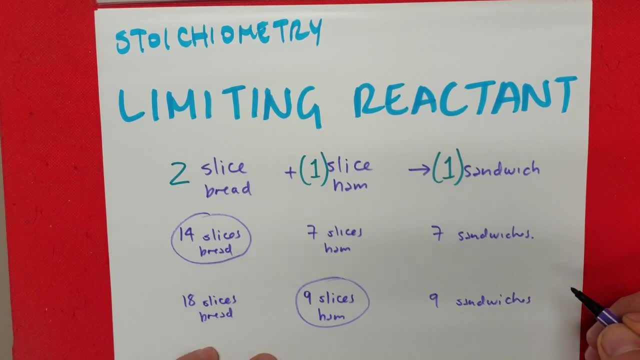 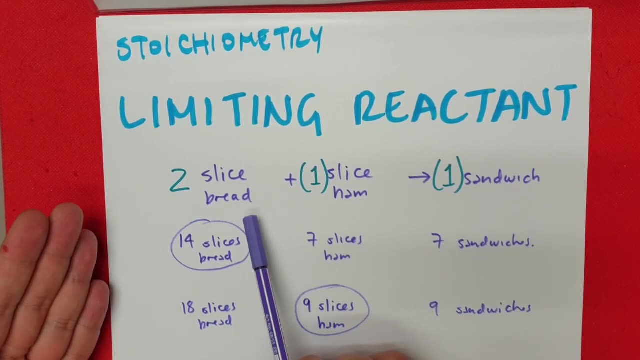 make 9 sandwiches. But just think about this. in reality, This would not be possible. We can have the 14 slices of bread, we can have the 9 slices of ham, But if this is our formula, where we're being asked to make a sandwich with 2 slices of bread and 1 slice of ham, 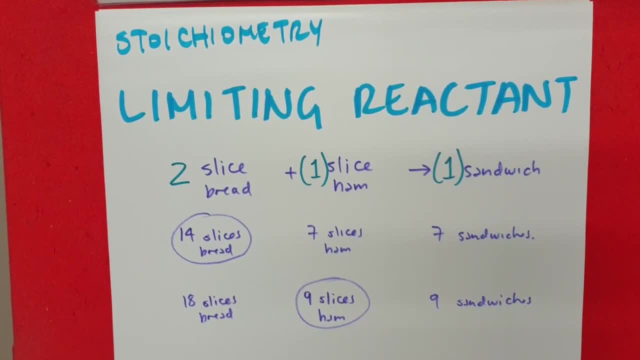 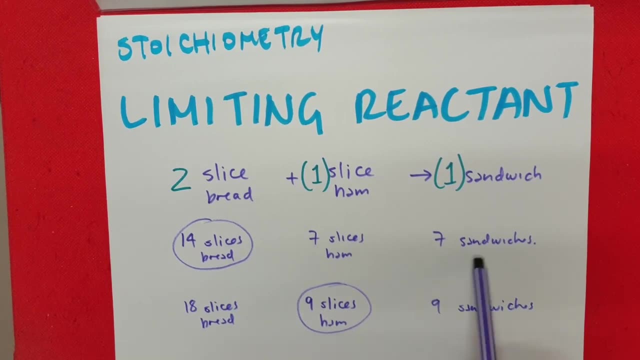 it's either this one or this one. So now we analyze the numbers and we say: wait a second, If I have 14, I need 7.. Do I have them? I do I do have them. So this is possible. But 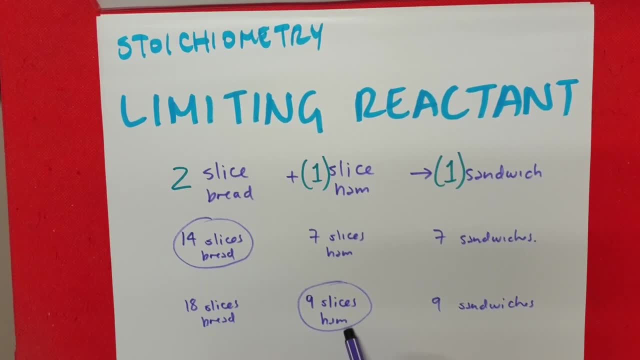 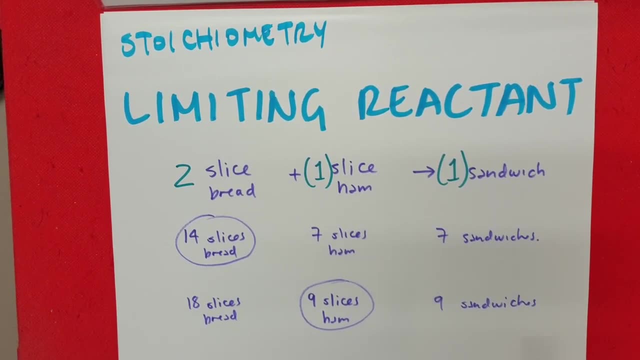 let's look at the second line. If I have 9 slices of ham, I need 18 slices of bread. Do I have them? I don't have them. So this one's possible, This one's not possible. So the actual ingredient that's holding us back from making more sandwiches. 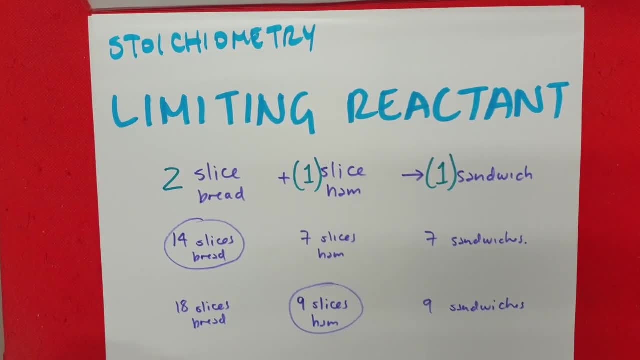 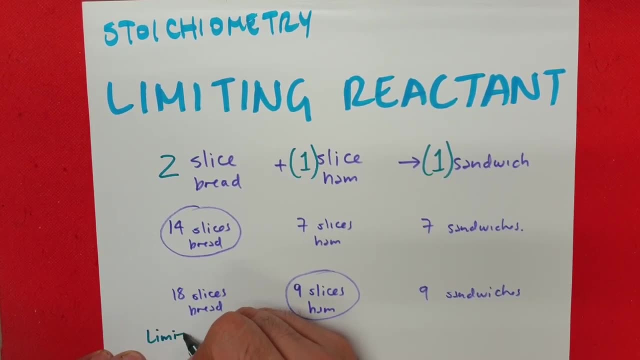 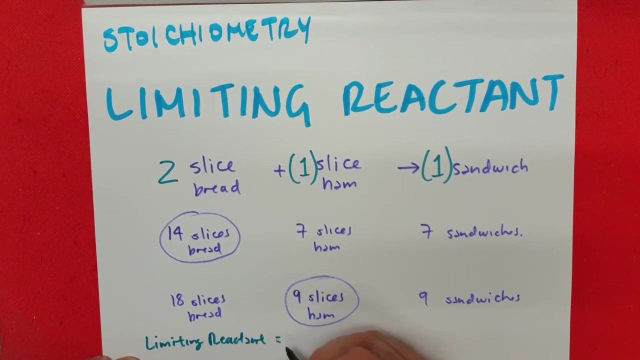 because we don't have enough, is the bread. So in this case, for this little exercise I'm plotting right here, our limiting reactant or limiting ingredient is the bread, Because we don't have enough bread for all the ham that we have, So is bread. And just as there's. 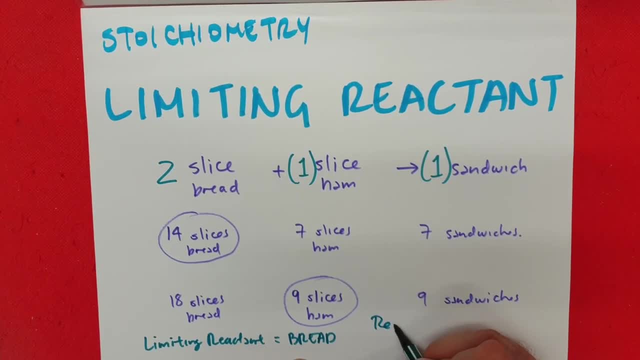 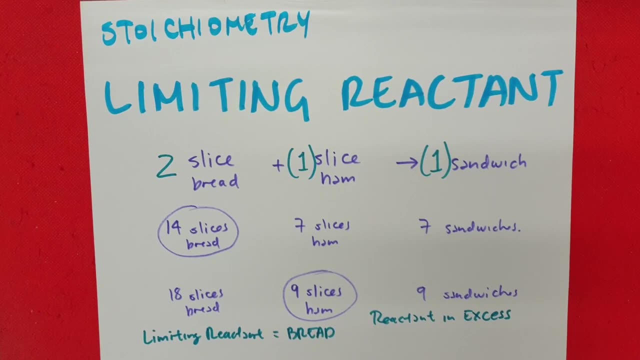 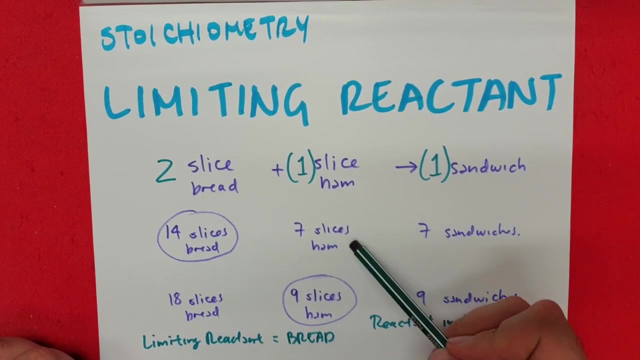 a limiting reactant, there's a reactant in excess, And in this case the reactant in excess is obviously ham. How do we know that the ham is a reactant in excess? Because we need 7 of it, which we calculated theoretically, and we have 9.. So we're going to have 2 slices of ham left over. 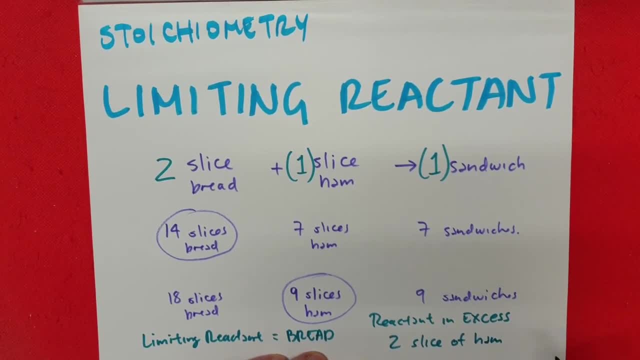 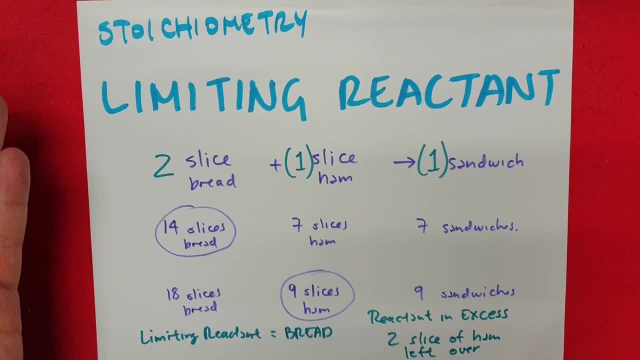 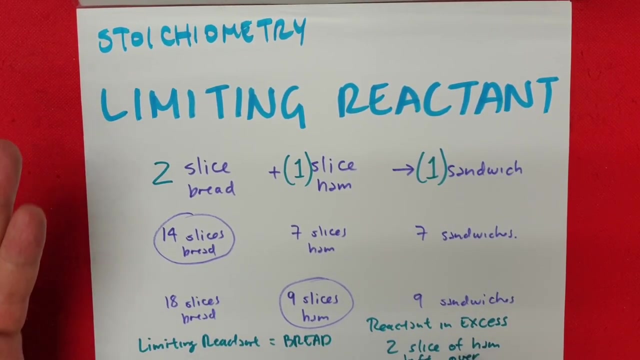 Left over. So in this case, a very simple question would be: you're given 14 slices of bread and 9 slices of ham. What is the limiting reactant, What is the reactant in excess, And how many sandwiches are you going to be able to make? 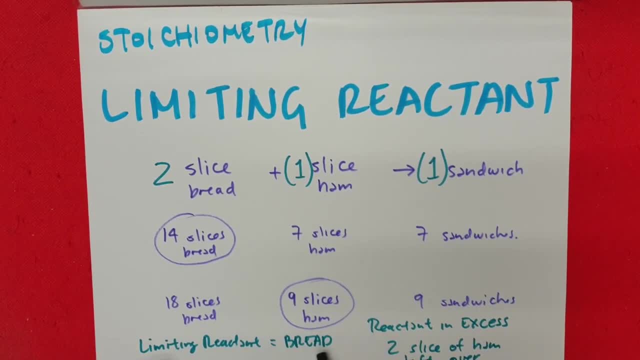 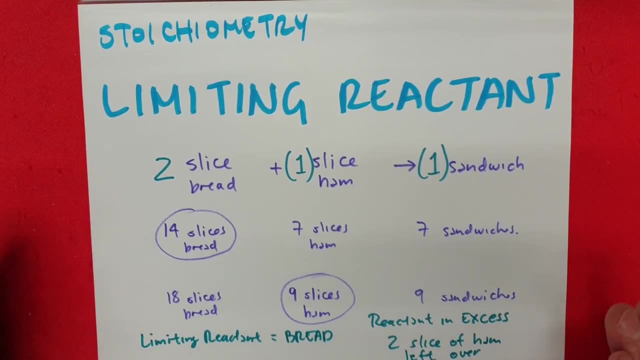 So we already answered this. in this analysis, The limiting reactant is bread, The excess reactant is ham. There's going to be 2 slices left over, And we know that the full amount of sandwiches that we're going to be able to make is 7 sandwiches according to this recipe. 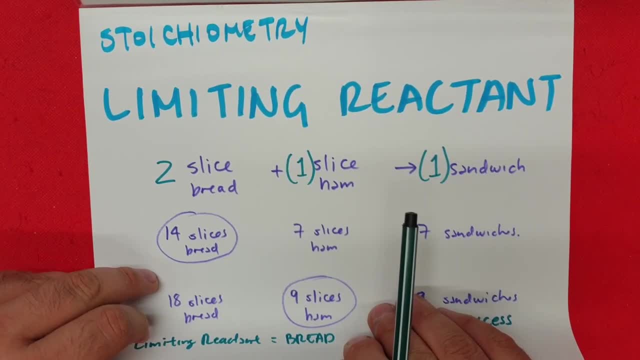 So that's a very basic explanation. If we want to make it a little bit more complicated, we're going to have to make it a little bit more complicated. If we want to make it a little bit more complicated, we're going to have to make it a little bit more complicated. 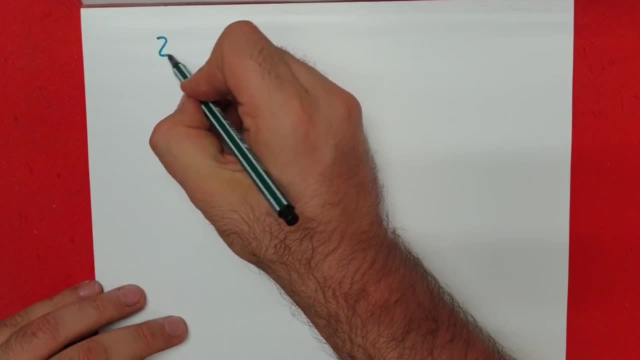 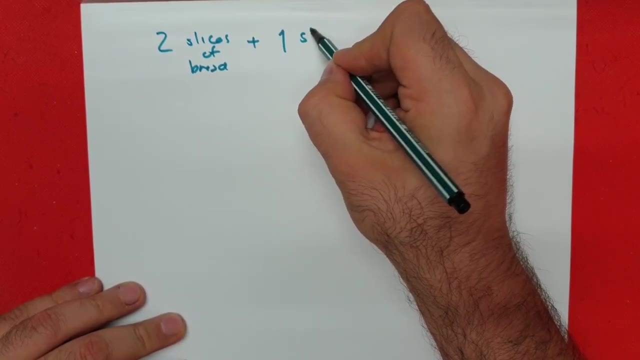 If we want to make it a little bit more complicated, we're going to have to make it a little bit more complicated. Let's use that same reaction that we created with the slices of ham. So 2 slices of bread plus 1 slice of ham is going to give us. 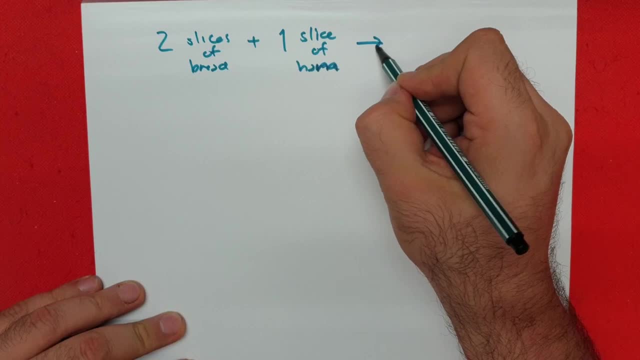 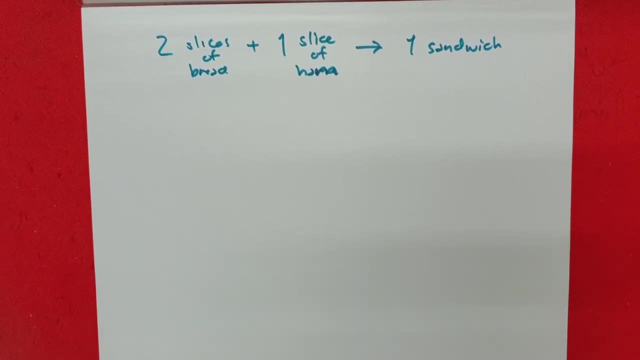 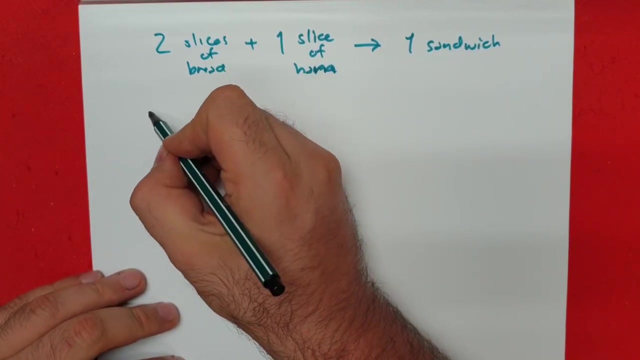 I don't know why I wrote ham. Ham is going to produce 1 sandwich, right? So we thought it was going to be this simple, but usually what happens is we're given the quantities in grams, So let's say that they give us. 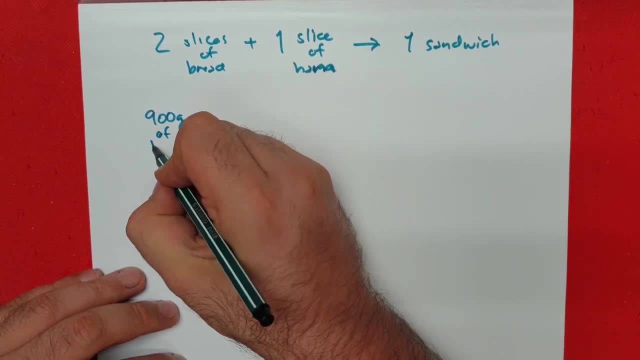 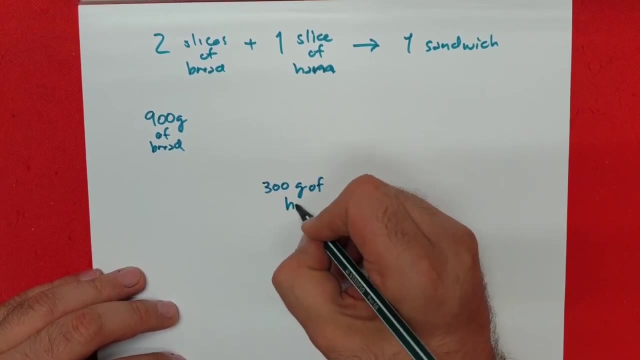 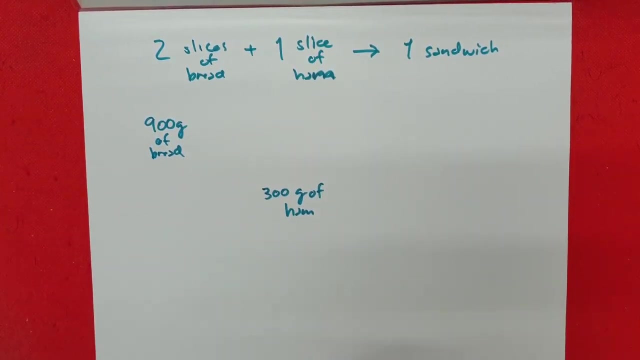 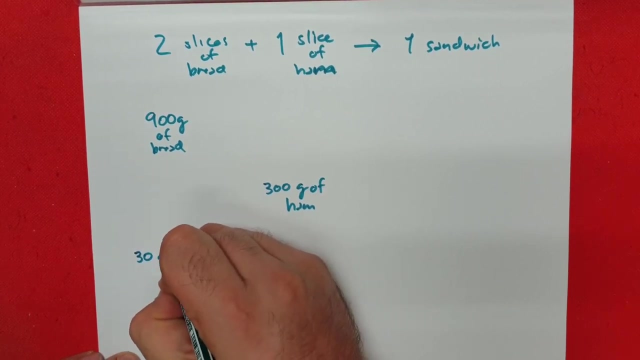 We have 900 grams of bread and we're given 300 grams of ham. Whoa well, we don't really know how to use it with the formula, because we would have to have some sort of equivalent. So in this case, let's do something really simple and let's say that 30 grams of ham equals 1 slice. 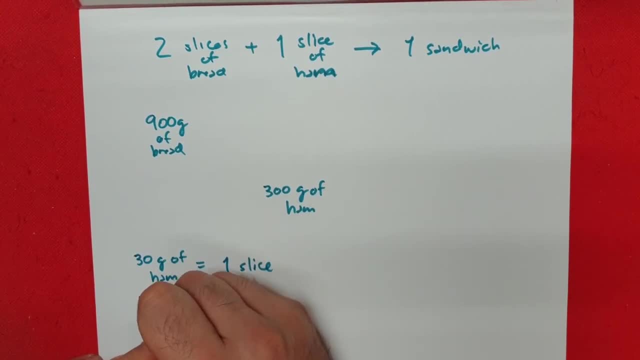 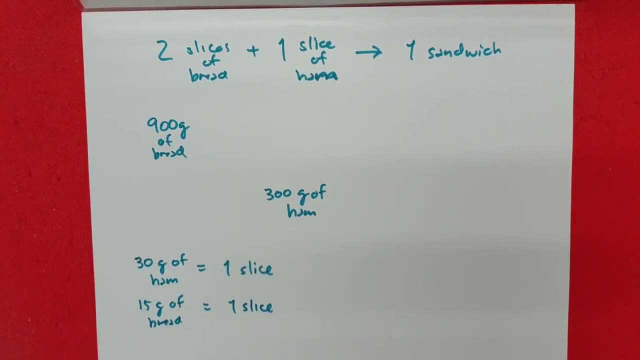 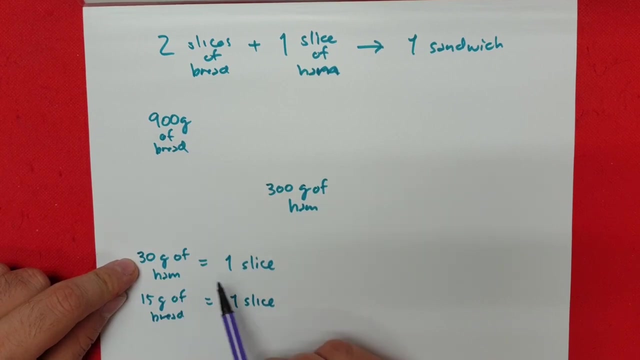 And 15 grams of bread equals 1 slice of bread. So now we can convert this right. So it's a very simple mathematical exercise. If we have 300 grams of ham and there's 30 grams of ham for 1 slice, this means we have 10 slices. 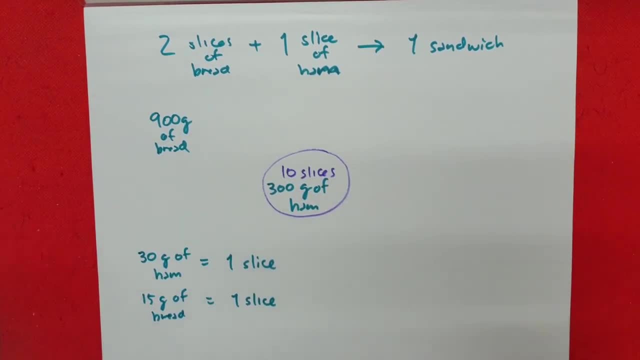 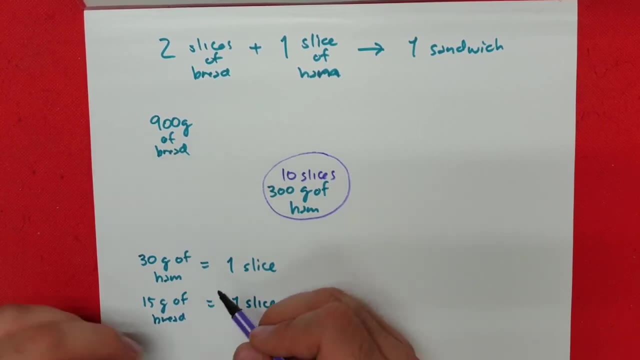 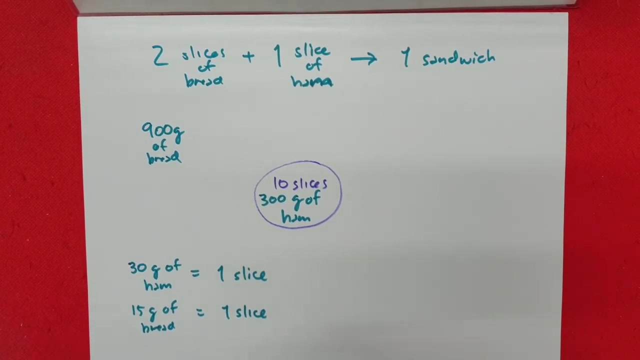 And I'm going to circle this because this is what we have. Okay, this is what we were given. And then, if 15 grams of bread equals 1 slice, 15. Can go into 900.. Let's see, 900 divided by 15 gives us 60 slices, which is also what we have okay, of bread. 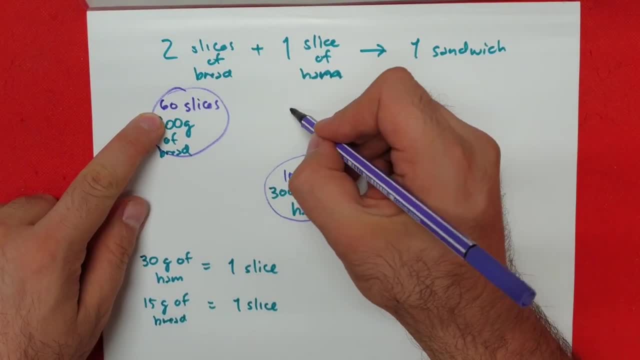 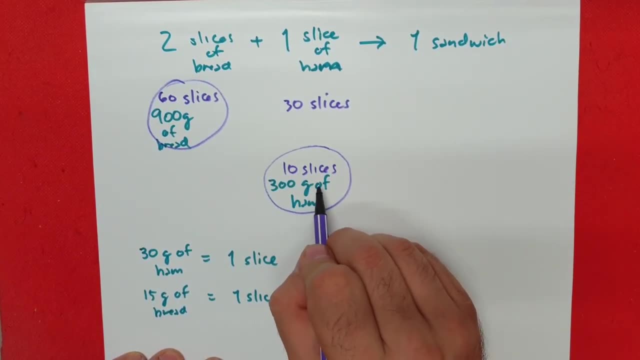 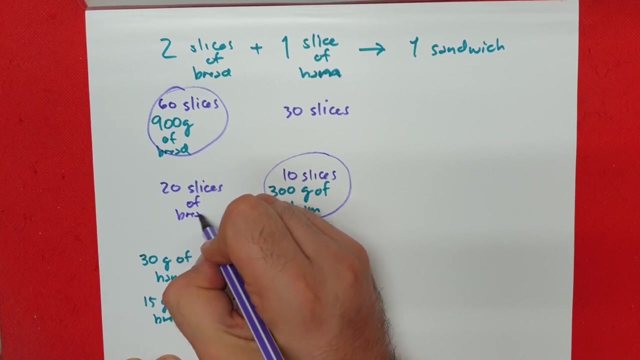 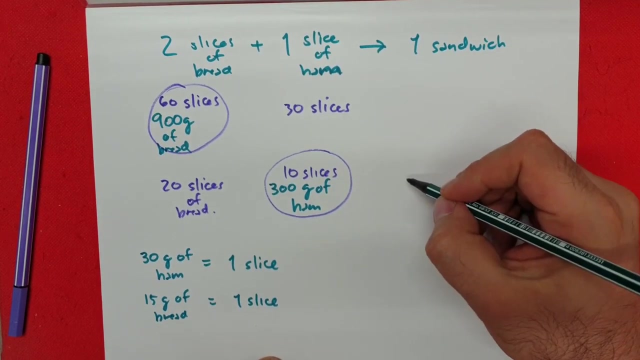 Now, if we have 60 slices of bread, it means we need 30 slices of ham, And if we have 10 slices of ham, we need 20 slices of bread. Okay, Okay, Okay, Okay. Now we do our comparison and we answer the three basic questions, which are: how much? 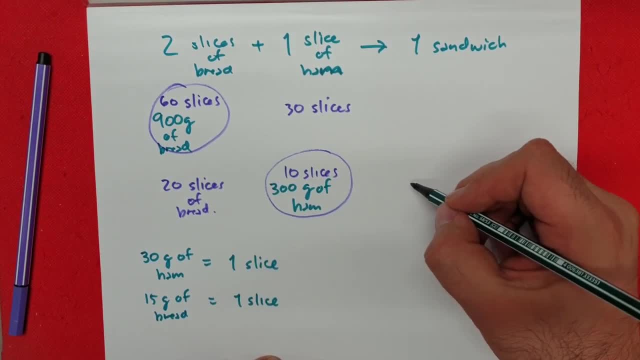 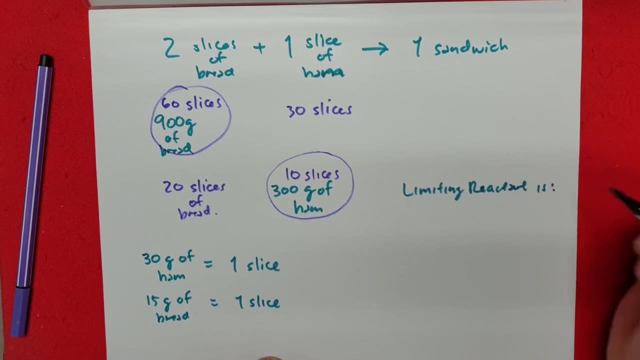 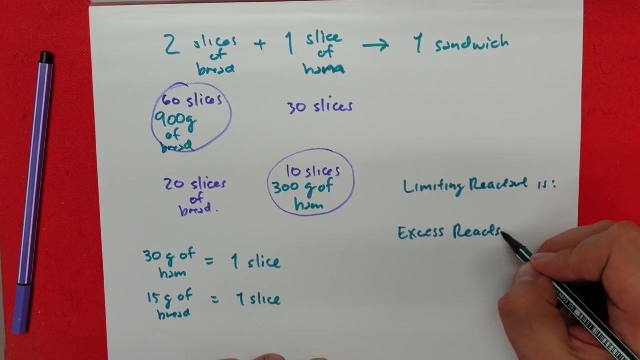 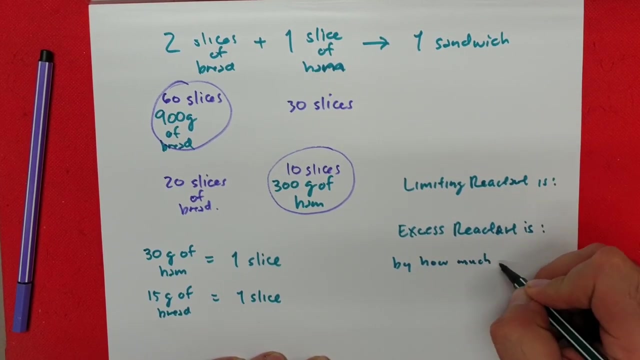 Not how much. Let me think about this really quickly. We would ask: what is the limiting reactant? So the limiting reactant is the excess reactant, Reactant Reactant, Reactant, Reactant Reactant, And is by how much? 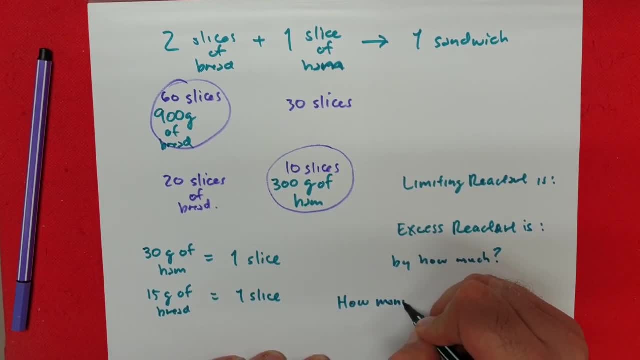 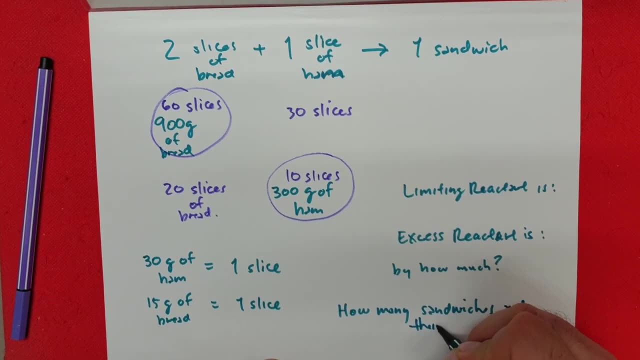 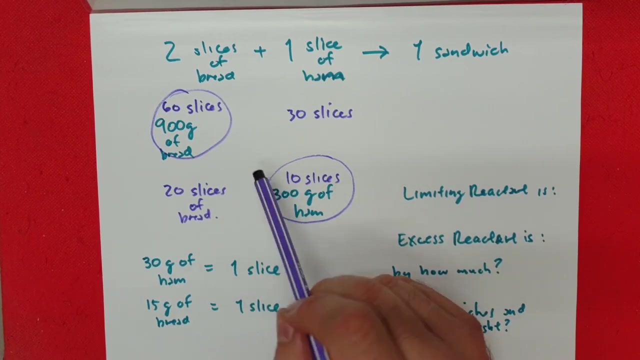 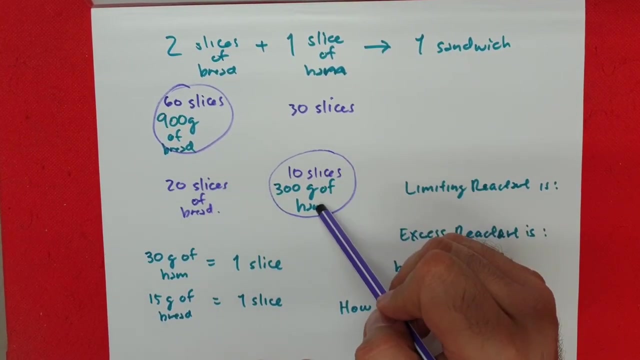 And finally, how many sandwiches and their weight, Uh huh. So when we look back at this, we can say: okay, we have 60 slices which we converted and we would need 30. Do I have them? I don't have them. I don't have those 30 slices. 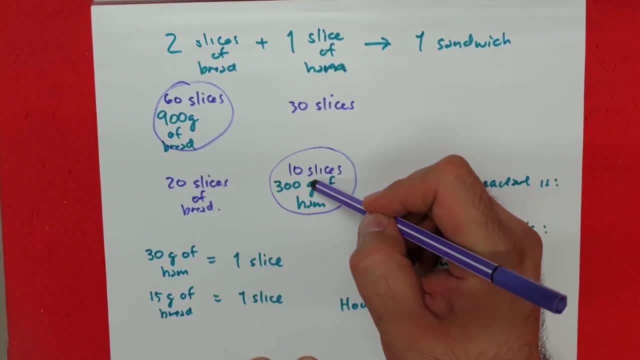 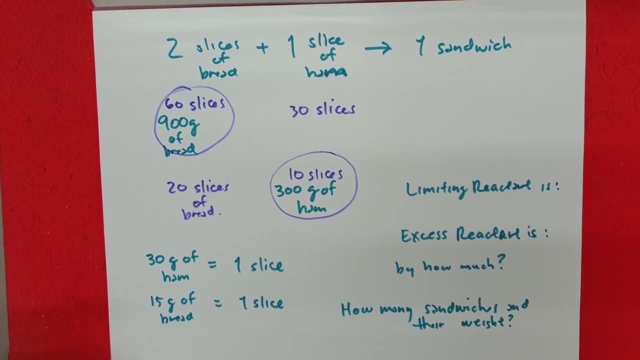 I only have 10.. If I have 10 slices, I'm going to need 20 slices of bread. Do I have them? Yes, I do. So a simple way to answer this is: let's look at our excess reactant. If we use 10 slices of bread, we're going to need 20.. 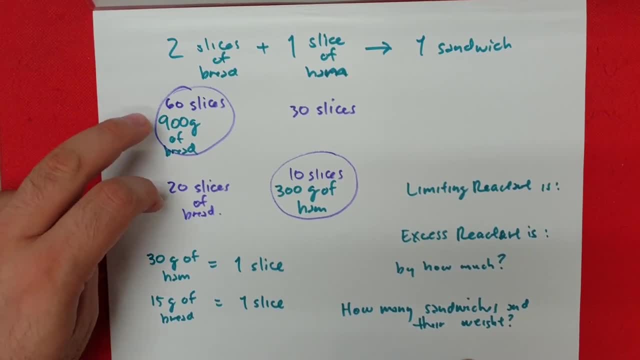 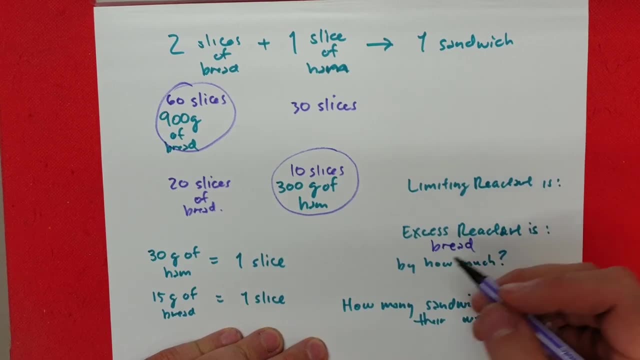 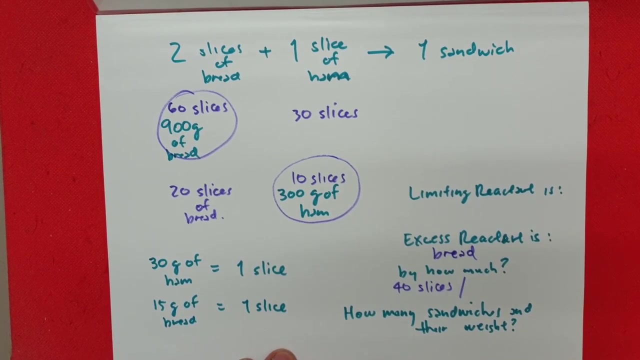 Do we have them? Yes, we do. And what happens? This is our excess reactant. So the excess reactant is going to be bread. And by how much? By 40 slices. And if we're very specific, 40 slices times 15, which is how much. 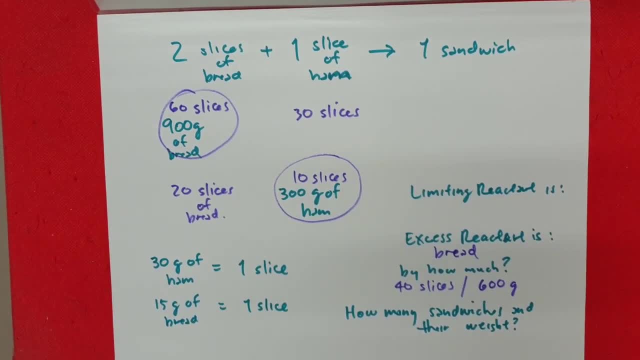 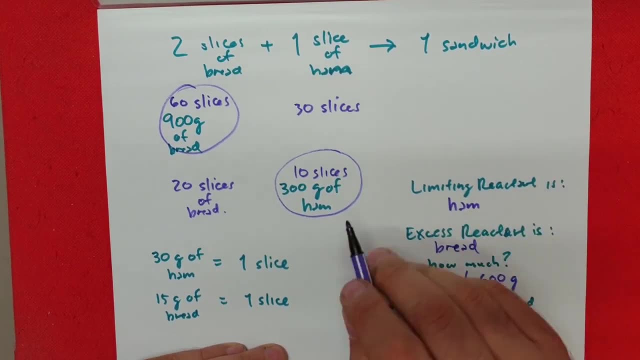 600 grams is going to be left over. So there's going to be a lot of bread left over. So if bread is the excess reactant, the limiting reactant, of course, is ham, which we already proved. So if ham is the limiting reactant and is the one we have, we're going to follow this.